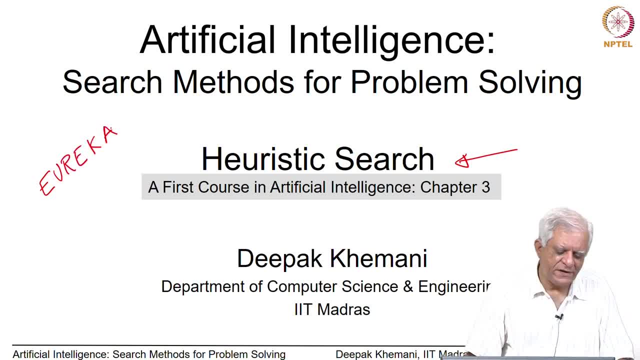 Greek word, The word heuristic, or the decrease in the weight, is equal to the weight of the water that is displaced. So once he realized that, he ran saying Eureka, Eureka And Eureka basically meant I know, I know, And the word heuristic also comes from the same source, which means 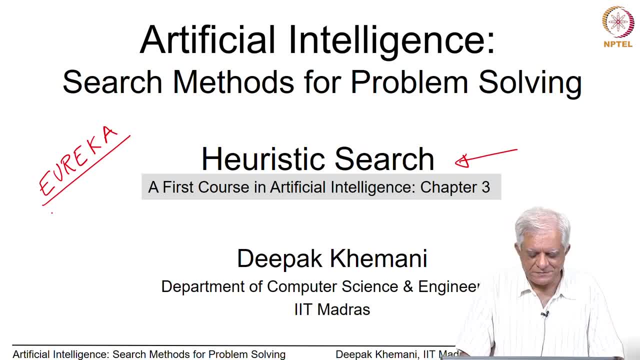 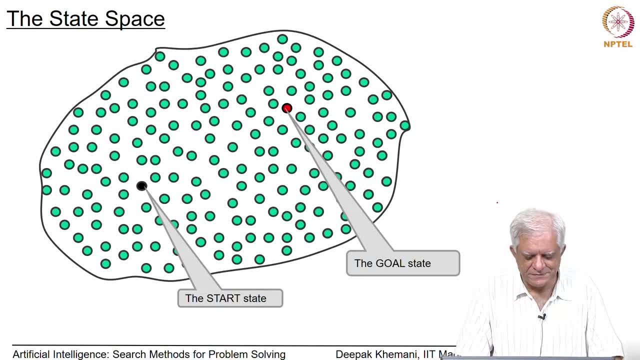 that in some sense, the algorithm knows where it should go. If you are following my book, you will find all the material on chapter 3, essentially. So let us just do a quick recap. We have a state space in which we have a start node. 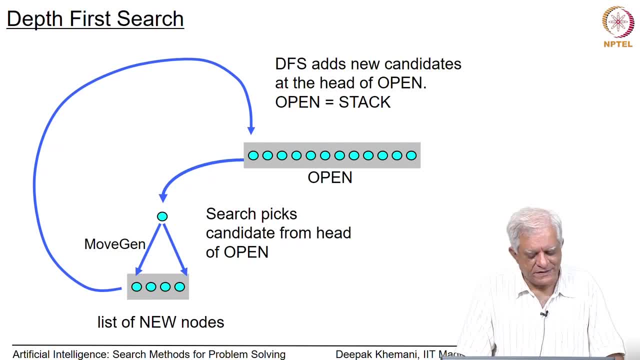 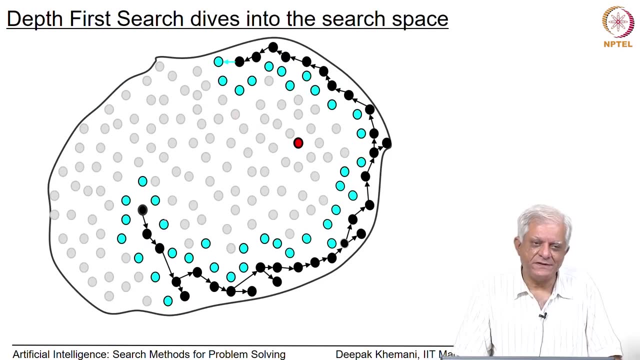 and a goal node and we have studied depth first search where we take out the nodes from the head of the list and then we add the new node back at the head of the list, which results in this behavior of depth first search that we have seen, that it dives into the search. 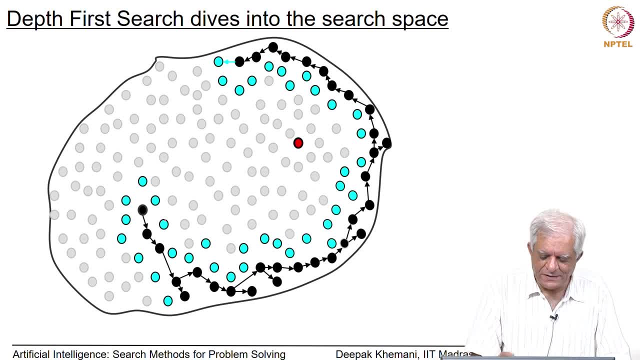 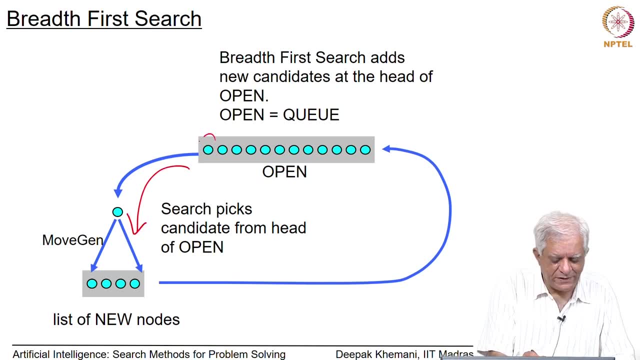 space. it has a very impetuous nature. It just goes off without you know. looking here and there, The other algorithm that we saw was that we again take out node Nodes from the, from the head of the open list, but this time we add them to the tail of the list and 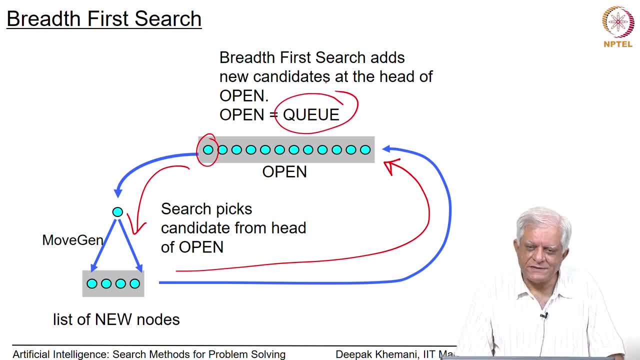 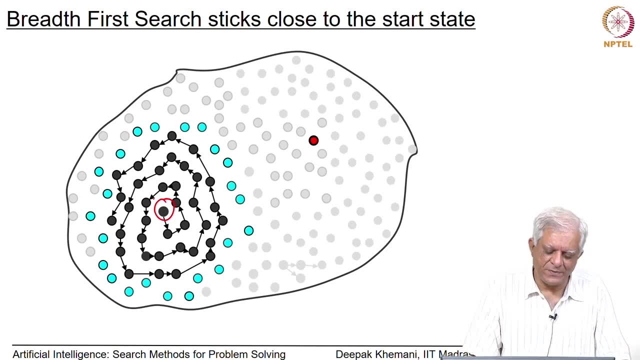 therefore, we treat open as a queue and, as a consequence, the behavior of the search algorithm is startly different. It tries to stay as close to the source node as possible, and you can think of it as a conservative search algorithm. and as a result of its 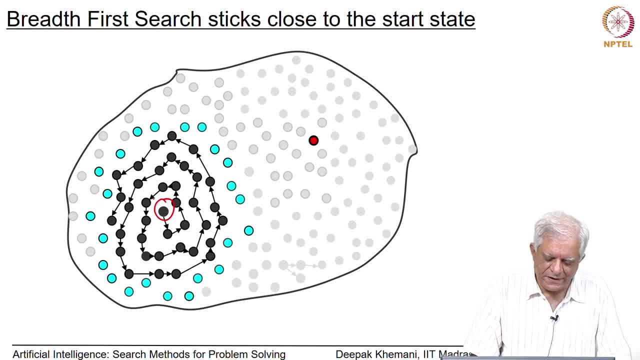 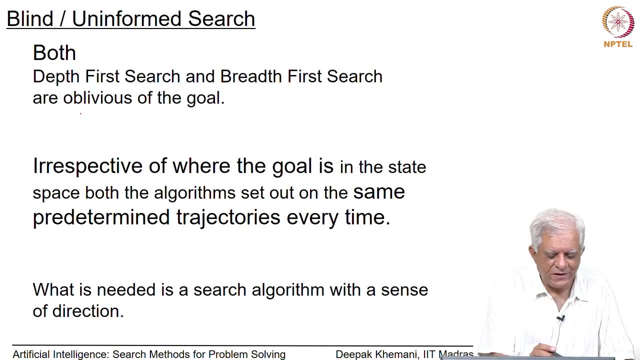 conservative behavior. it also gives us the shortest path, which means the least number of moves in the solution. Now, both of them are oblivious of the goal. They are just not aware of where the goal is- Ideally the goal they should try to move. 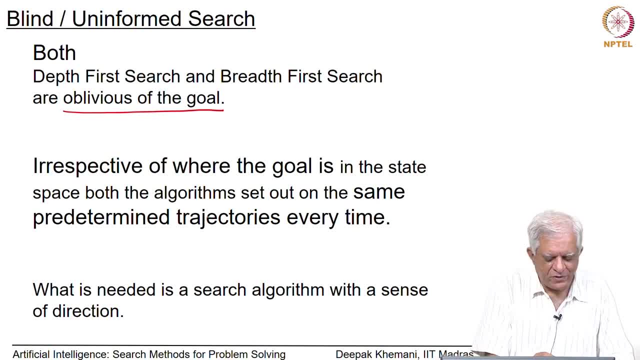 towards the goal. So, irrespective of where the goal is, both the algorithms follow the same predetermined trajectories every time. Now, obviously that is not intelligent behavior, but it could still form the basis or a foundation layer of a higher level algorithm which uses them. but even for this, 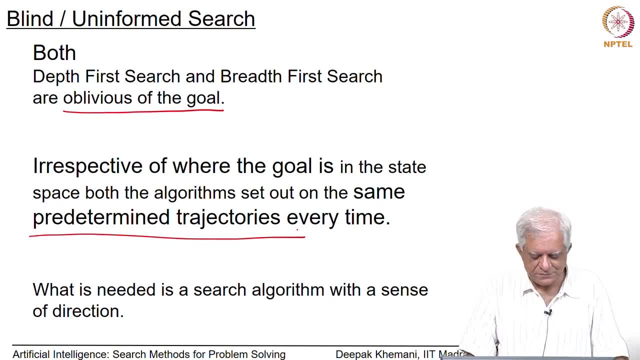 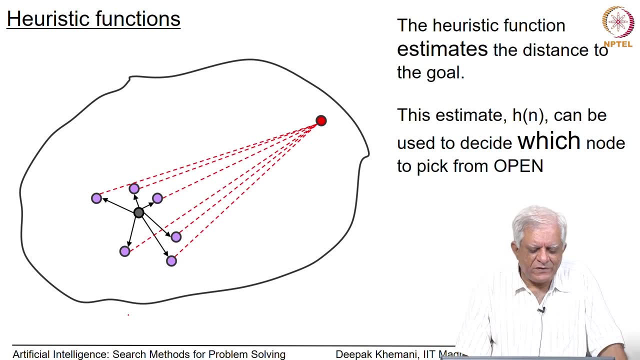 basis or foundational algorithm. we can try and do better, So what we need is a algorithm with a sense of direction, and that is what we will start looking at in this sequence of lectures. So we have a notion of a heuristic function, The heuristic function, which is a function. 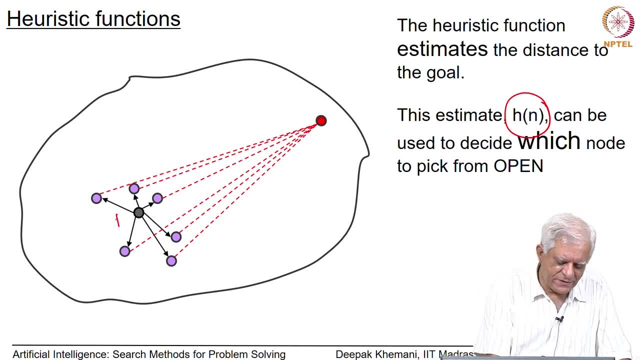 of a node n. In this case this is the node n. Let me draw that again. n. Traditionally we write it only as a function of the node n, though in reality it is a function of the node n and node g or the goal node. but since very often you may not specify a goal node, as we. 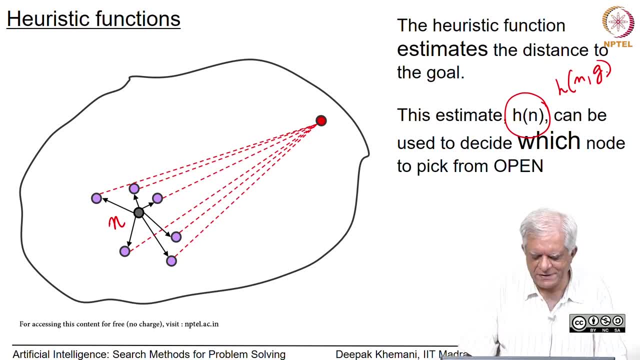 saw in the water jug example a little bit earlier, You may specify the conditions for the goal to be true, which may be true in a set of nodes. So we do not tend to express that goal part here. and it is kind of implicit that what the heuristic function does is that it estimates. 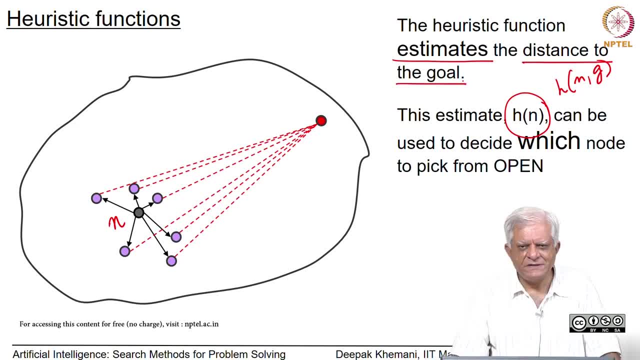 the distance to the goal, essentially For sake of simplicity. in this diagram we have drawn one goal, but if there were many goals, then for each node that we are interested in, we would choose the distance to the nearest goal, essentially So, as n varies over these. 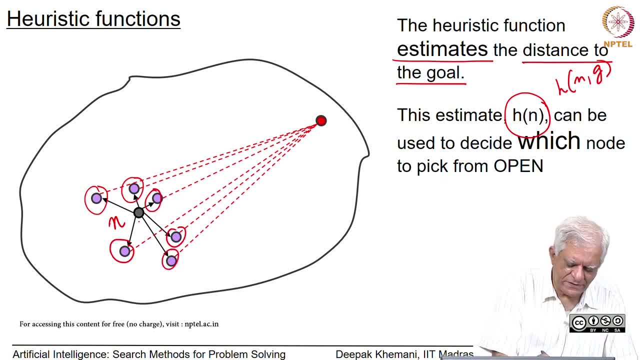 different nodes we can, which are the successors of that start node s. we can compute the heuristic value and then, based on the heuristic value, we decide which node to open, Unlike depth- first search and breadth first search, which always shows the nodes in a 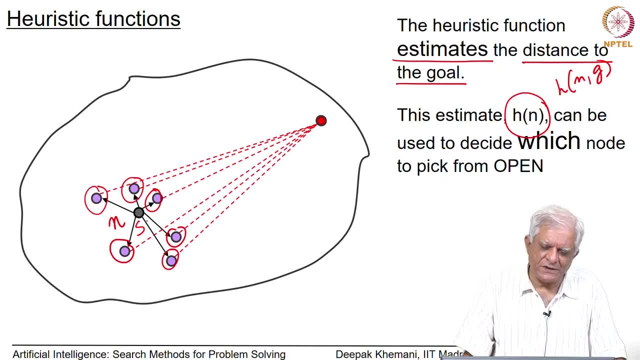 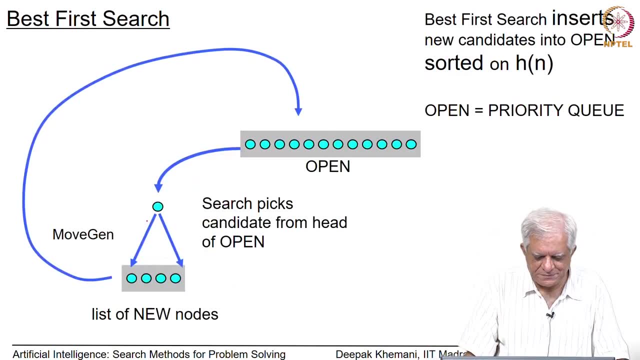 predetermined fashion. So heuristic search will choose the nodes based on the estimated distance to the goal, and that is why it is called a heuristic search algorithm. The algorithm that we are talking about will be called best first, in the sense that it always chooses the best node first. 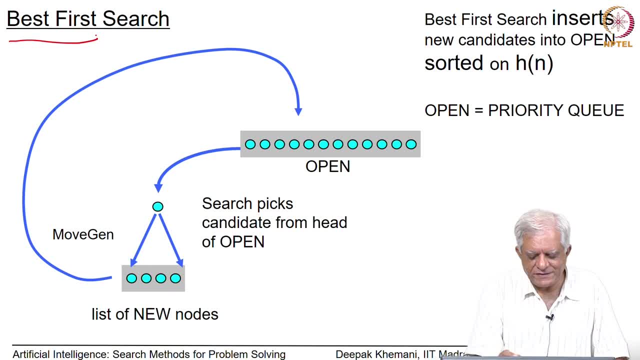 Now, essentially, you can imagine that you have a set of candidates which are stored in the open list. For every candidate, we know what is the estimated distance to the goal and we want to choose the one which has the lowest estimated distance to the goal. The way to implement this, which? 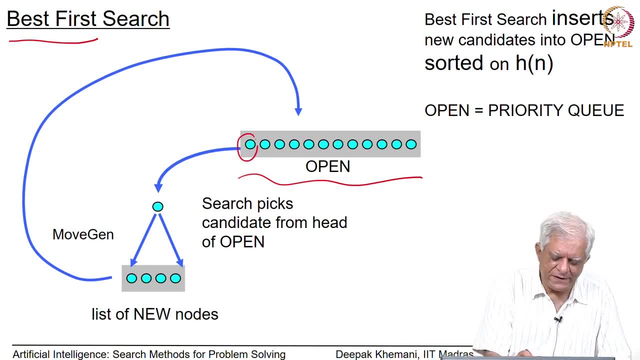 is consistent with what we have done earlier is that we will still extract the node from the head of the open if it is a list like this, but we will keep this open sorted on the heuristic values. Sometimes these are called as h values, So this open list will be shortest on the h values. 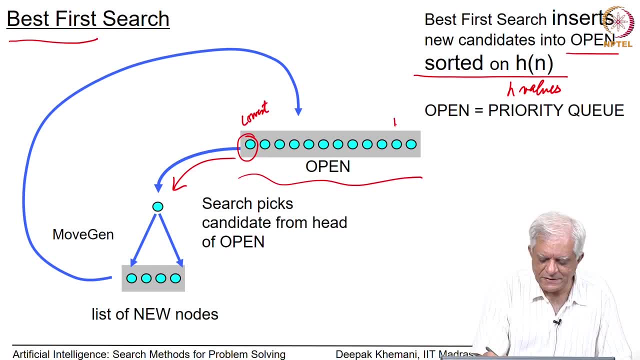 so the lowest will be here and the highest will be here. So when we pick the node from head, it will always pick the one with the lowest h value and when we are done generating the new nodes, we will insert them at an appropriate place. essentially, 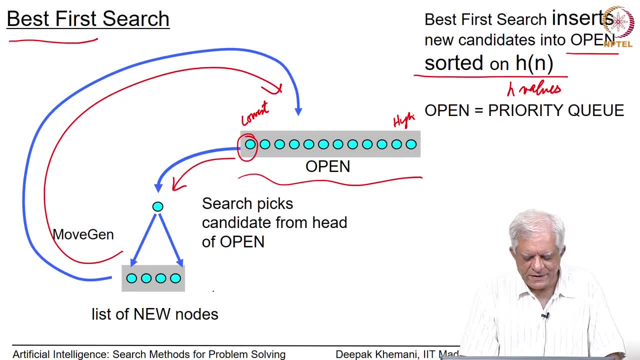 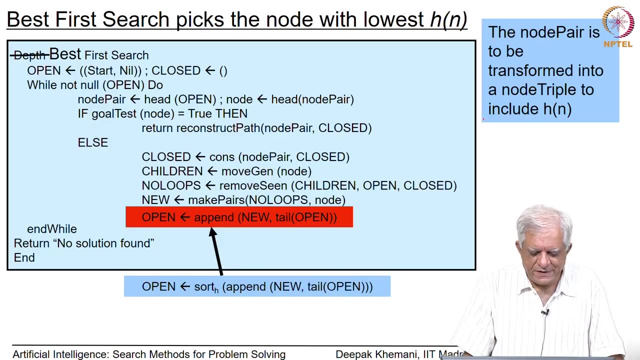 In practice. of course, we do not sort the list In practice. we would maintain open as a priority queue, which is just an efficient way of making sure that you always extract the node with the lowest heuristic value, essentially. So here is a variation of our algorithm that we had written for depth: first search. 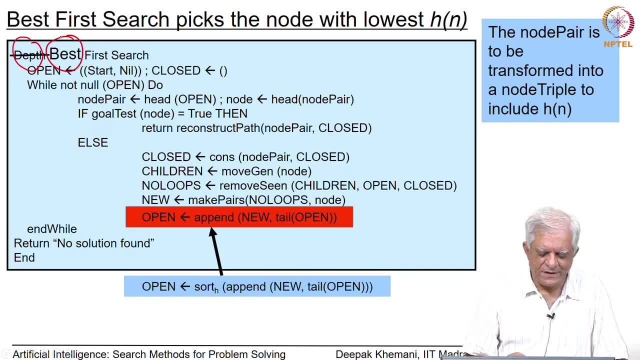 So we are not doing that first search, but we are doing best first search. The only difference that we are, only difference that we are doing here, is that instead of saying that you are going to append the new nodes to the tail of open, we are saying we will do that, but after that. 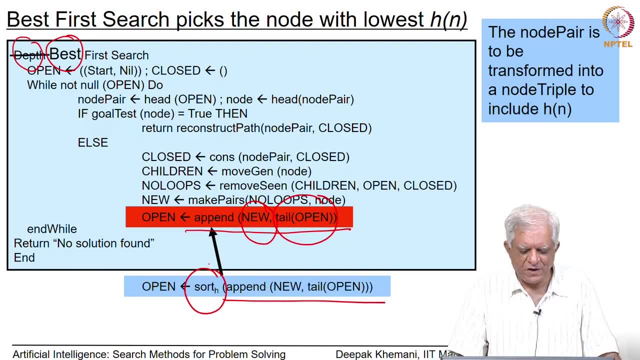 we will sort the nodes on heuristic value. Of course, a little bit of extra change that we also need to do is that instead of the node pair we will have to make it a node triple and include the heuristic value as part of the node representation. So in the 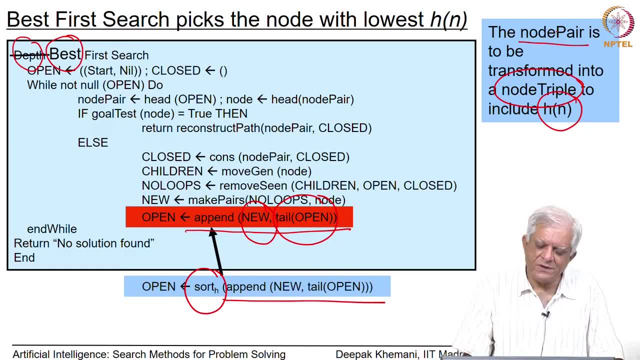 node pair, we have the current node and the parent node. In the node triple, we will have the current node, the parent node and the heuristic value for the current node. essentially So, as I said a little while ago, in practice actually open is maintained as a priority. 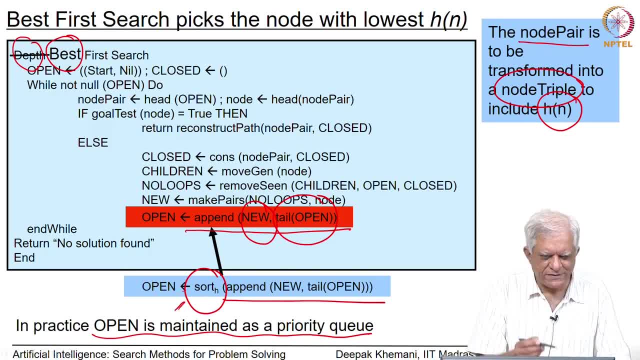 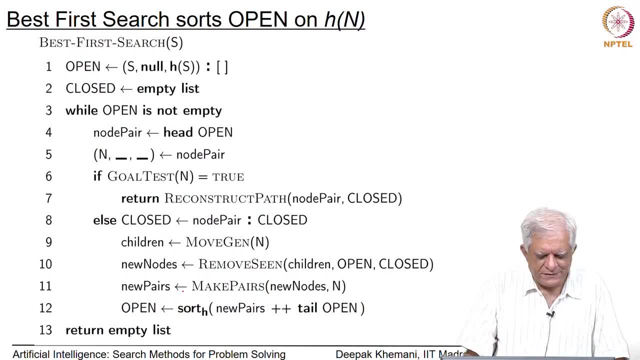 queue, but we can conceptually think of it as being sorted essentially, which is doing the same thing, that always giving to us the node with the lowest heuristic value. If you were to do this, then we have our modified algorithm. best, first search here and observe. 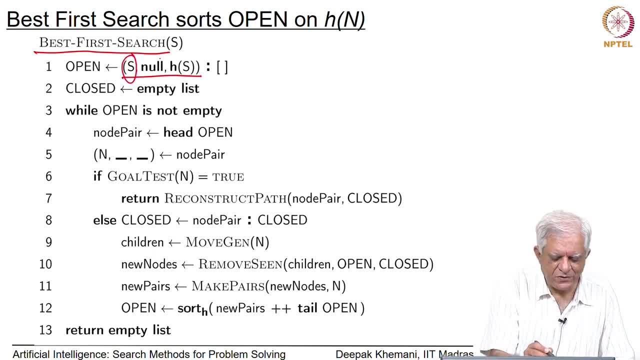 that we have a triple here, where we have a start node, it has a parent, which is null, and the heuristic value of the start node, which is the estimated distance to the goal. essentially And at every point, we extract a triple, and the first node, n, is what we are interested. 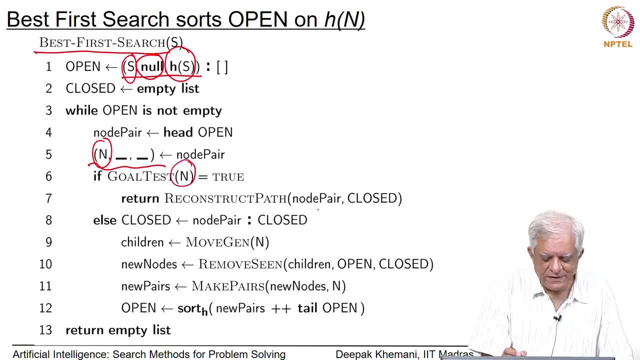 in. we apply the goal test to that n, and again we have called this node node pair here. this is simply for the sake of reusing the earlier code, but we could have called it node triple after all. there is nothing in the name, essentially. 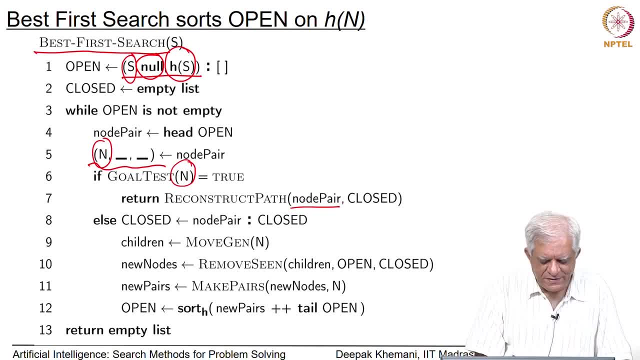 So everything else remains the same, that except that we have changed the representation to include the heuristic value. So there you go, and conceptually at least, we are sorting this open list, which I will again repeat to say that in practice you would. 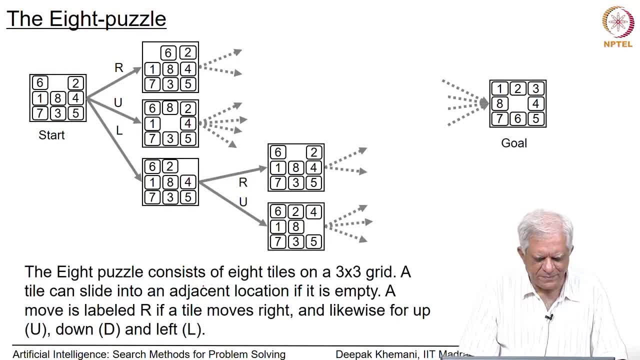 want to do it as a priority queue, which is implemented as the heap. Now let us look at this problem that we have seen earlier, the eight puzzle problem, in which you have to move around tiles. So either you can move this tile here or you. 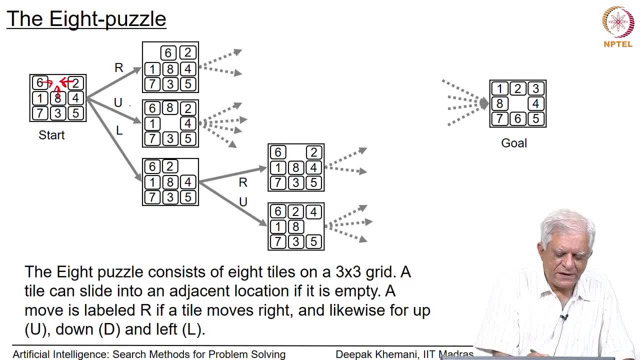 can move this tile here, or you can move this tile here, resulting in this three moves that we can see here, And then, once having made a move, you can choose. you have to choose again what is the next move you want to make, and so on. So the thing that we want to focus on is 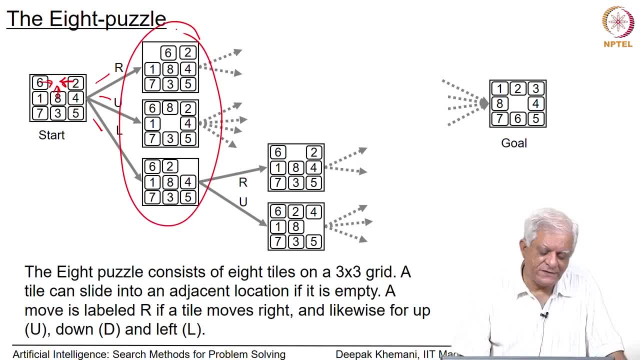 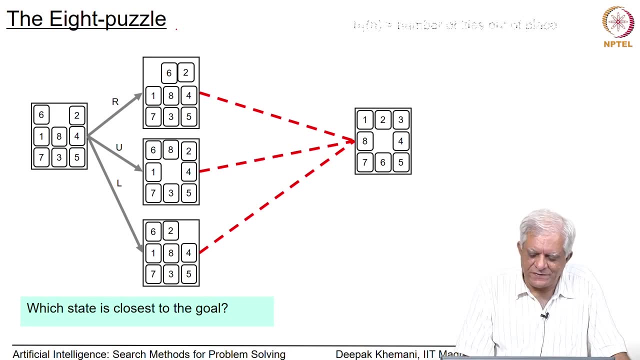 how do we decide that, for example, between the three of these nodes, what is the node that we should pick? How do you estimate the distance to the goal? essentially, So we can think of a couple of heuristic functions, One function which simply says: 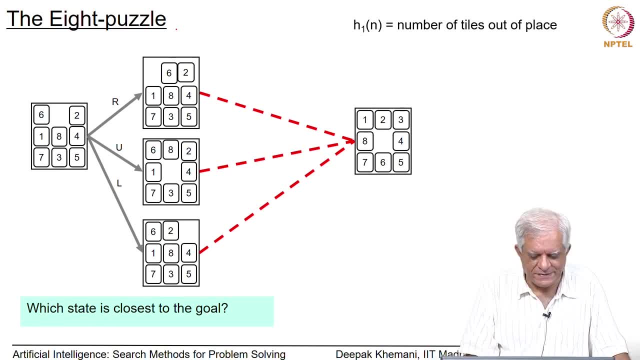 that count the number of tiles which are out of place. So if you look at this, for example, the first successor here- we can see that 6 is out of place because it should have been here. 2 is out of place because it should have been here. 1 is out of place. 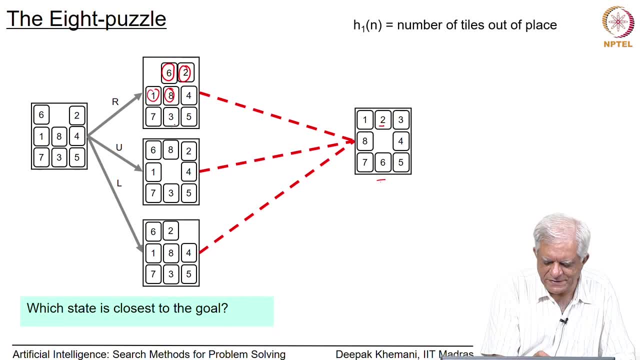 8 is out of place, but 4 is in place, 7 is in place and 3 is out of place, So you can see that 5 tiles are out of place. 3 tiles are in place, So we can think of this as: 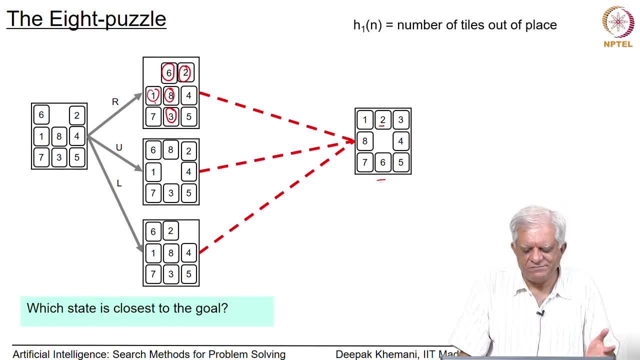 a distance of 5, which says intuitively that you have to change the position of 5, this thing, essentially, The other measure that we can use is the notion which is close to Manhattan distance. So both of the heuristic functions try to tell us which node is closer to the goal. 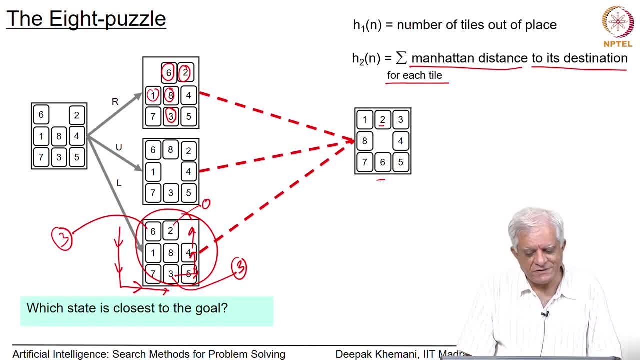 The first one is kind of more coarse because it simply says how many tiles we have to get into place. The second one is a little bit more refined because it tells you how much each tile will have to move to reach the goal. node, essentially, The trouble with heuristic. 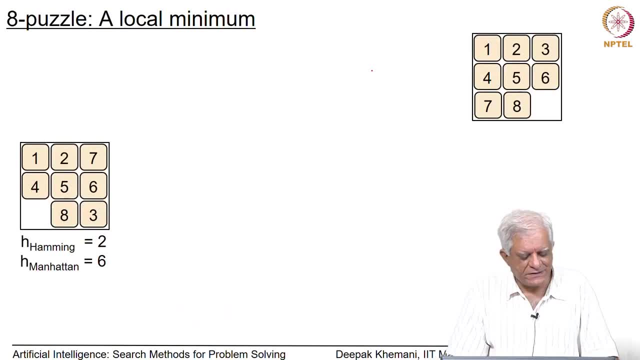 functions is that it is very difficult to define heuristic functions which are accurate. So here let us look at another function. So we are going to look at this example, where this is the node n that we are looking at, and you can see that the first heuristic function, which is also called the hamming 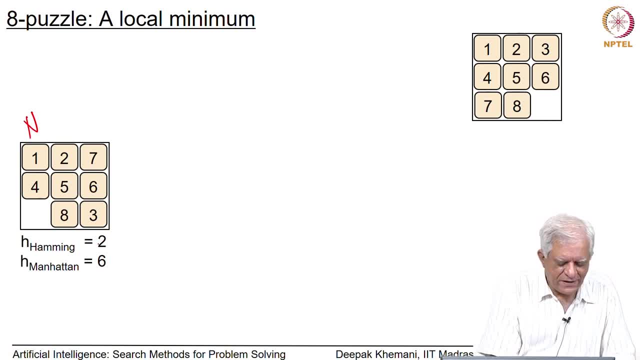 heuristic function because it tells you how many things are out of place. So in this case we can see there are two things out of place: One is in place, 2 is in place, 7 is out of place, 4,, 5,, 6 are in place, 8 is in place and 3 is out of place, So that 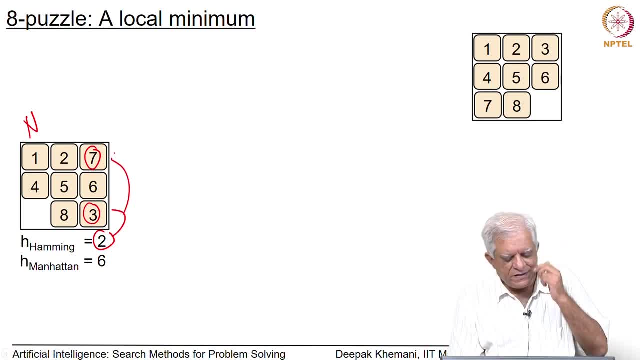 gives us this count of 2, essentially, If you had counted the distances, then this distance would be 6 for this node. Now, if you look at the 2 successors that this node has, you can move 4 down. that is what we. 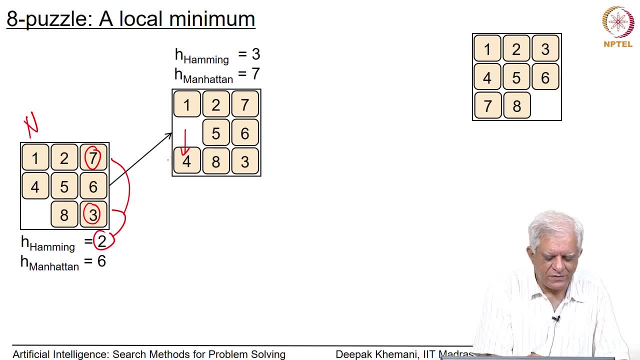 have done here and we get this thing, and now 4 was in place earlier and now it has gone out of place. So all these values have gone up by 1 here essentially. Alternatively, you could have moved 8 here in the second move and again 8 was in position and it is. 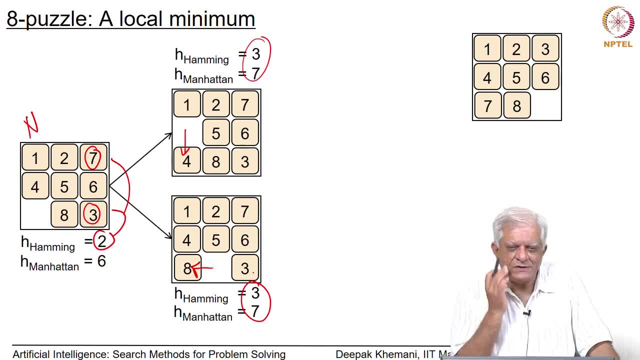 gone out of place, So the heuristic values have gone up. So this kind of illustrates the fact that heuristic functions are not always accurate. Now, clearly, if you want to go from this node n to the goal node g, you will have to go through one of these through. 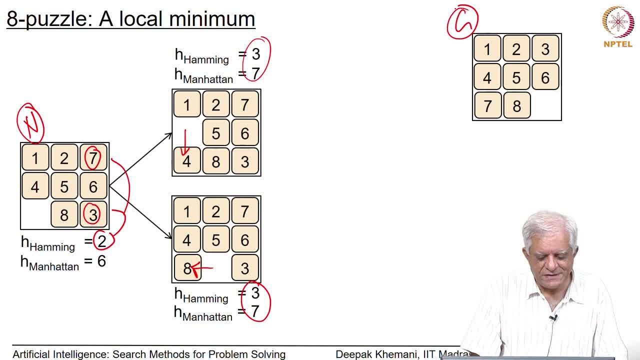 children node, but the heuristic function is telling you that both these children on both the heuristic functions, Other heuristic functions are worse than the current node and that is a phenomenon of local minima In this case. we will explore this a little bit more. That is a problem. 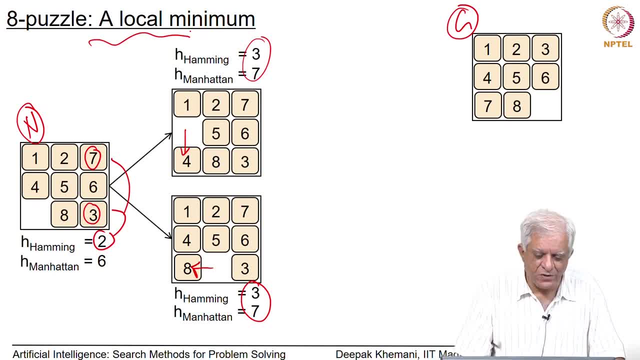 with heuristic functions that you often end up with local minima or maxima, where essentially what you want to reach is a value of 0, and you are starting with a value of 2 in the case of first heuristic function or 6 in the case of second heuristic function. but in 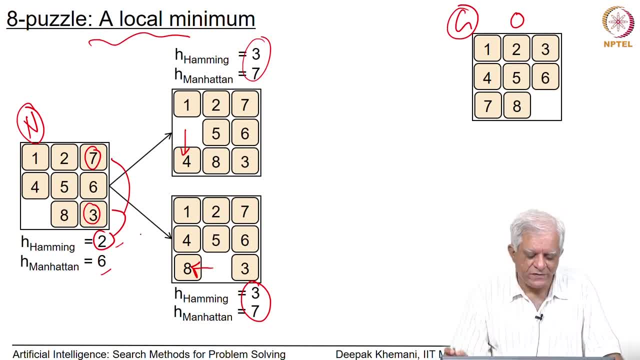 both the moves. the heuristic value is going up essentially, which does not look very encouraging, but it has to go through one of those nodes Very often. if you have played this puzzle as a child, you would have seen some pictures which are trying to, which are placed instead of this numbers. 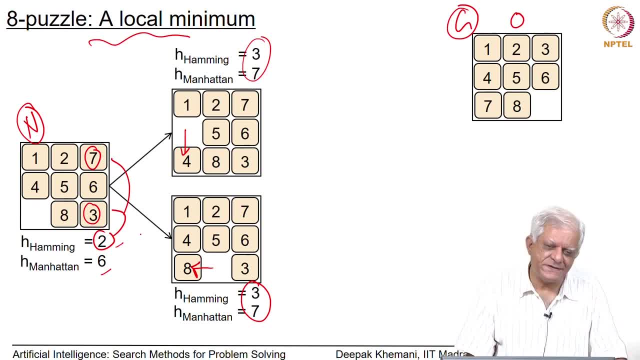 And in from that perspective we can think of this as a similarity- that you try to move to that successor node, that successor which is more similar to the goal node. ok, So in this example, either move increases the distance to the goal, but if you are working with a puzzle which had picture, 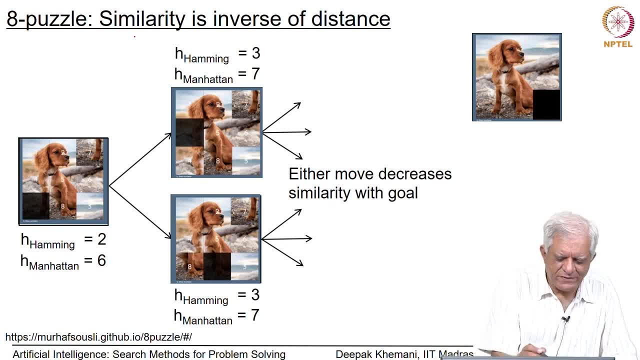 on it, then you can see that that the node n is more similar to the goal node g, then either of the two successors and you can think of similarity as the inverse of the distance, because the closer you are, the smaller is the distance, the more is the similarity. So 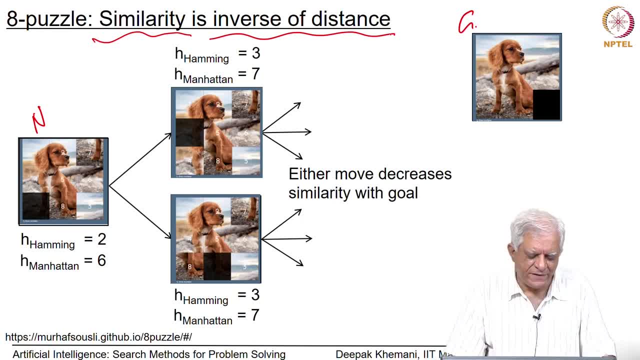 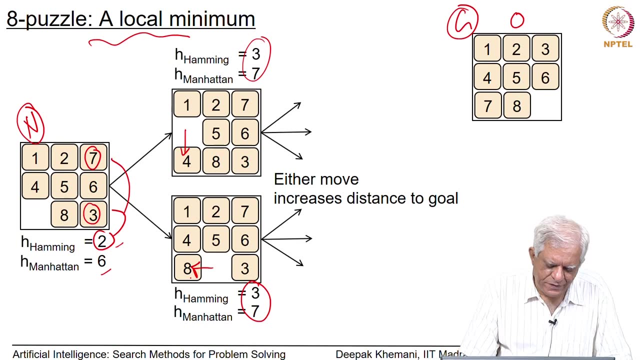 that is another way of looking at it and this also illustrates the fact that if you make either move, that, if you move this style here or if you move this style here, which is what we did in the same this thing, because it is the same puzzle actually, with the figures- 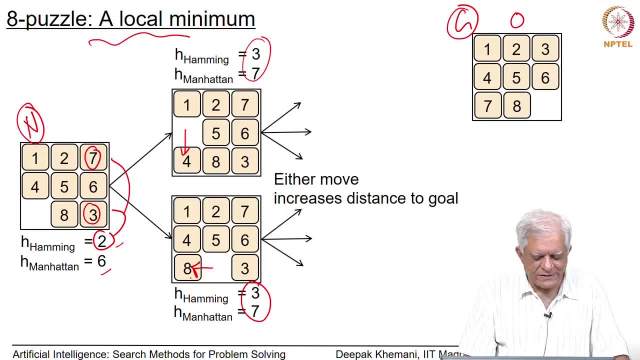 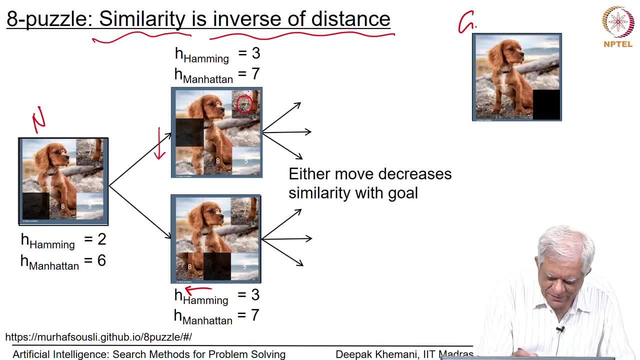 of the, with the picture of the dog thrown in the location, is still the same. if you, if you were to kind of look at this slide carefully, you would see the number that we were talking about: seven is here, eight is here, and so on. its its just that we have pictures, and therefore 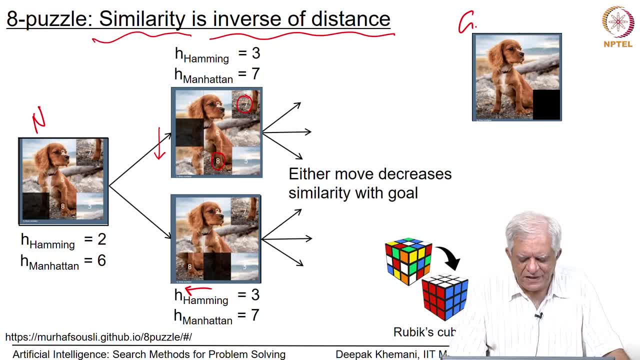 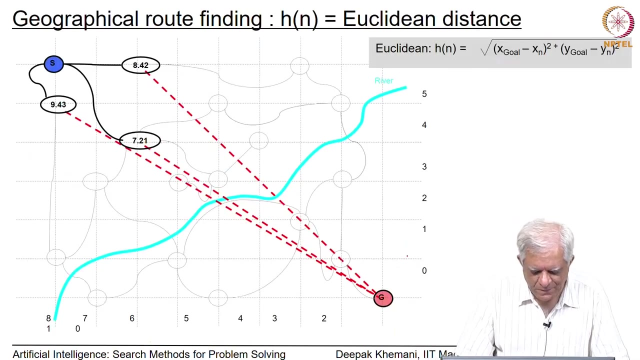 we can think of similarity 士. we can see similar phenomena for rub성을, space cube. some of you must have checked and solved is that very often you have to move from state which is fairly similar to the goal state. shuttle move makes it a little bit less similar. So this problem we will look at again later. 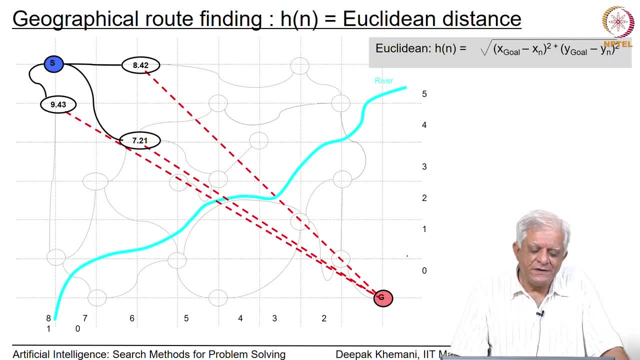 Here is another problem. Supposing you want to do geographical route finding, For example, Google maps does it for you nowadays- And the problem here is that you are at a start location here And from this start location you can either go to this successor or this: 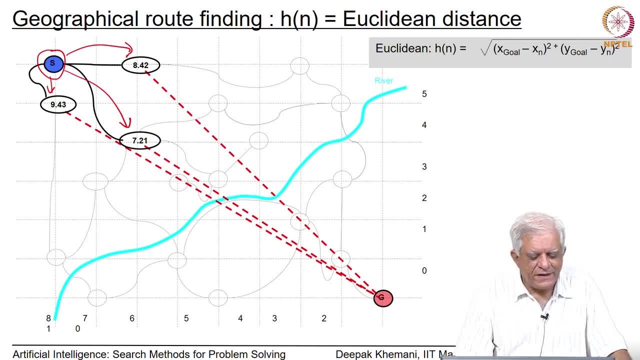 child, or this one or this one, And you have to choose which of those 3 is the right move to make if you want to reach this goal. node here. So this dash red line that you see, these are Euclidean distances, because the map is 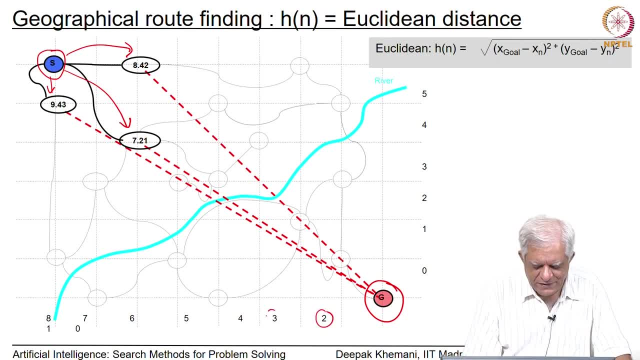 on a grid And you can see that. let us say this is in kilometers. So we are 2,, 3,, 4, 5 kilometers away and likewise in this direction, 1,, 2,, 3 kilometers away. 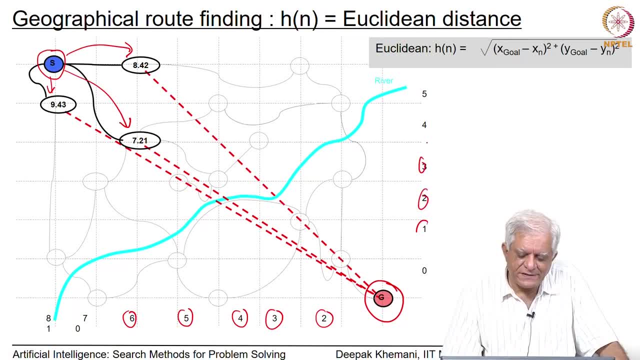 1, 2, 3 kilometers away. 1,, 2, 3 kilometers away. So one way of estimating the distance to the goal is to measure the Euclidean distance, which is the distance as the crow flies, which you know is the formula which you can compute. 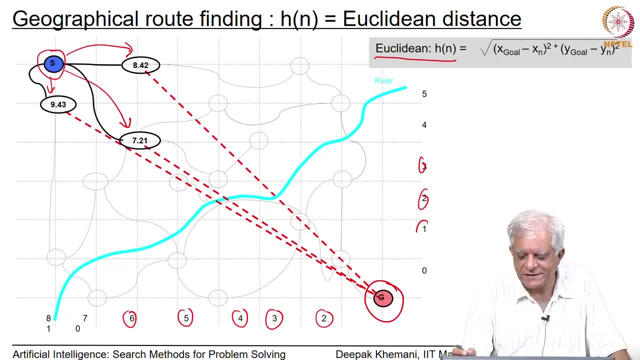 by taking the differences, adding and taking the squares of the differences, adding them and taking the square root, And this red lines that you see here essentially are the distances as the crow flies and the numbers you see inside this are the actual computed values. So 8.42, 9.43 and 7.21.. So, clearly, this is the best move to make for you and you can. 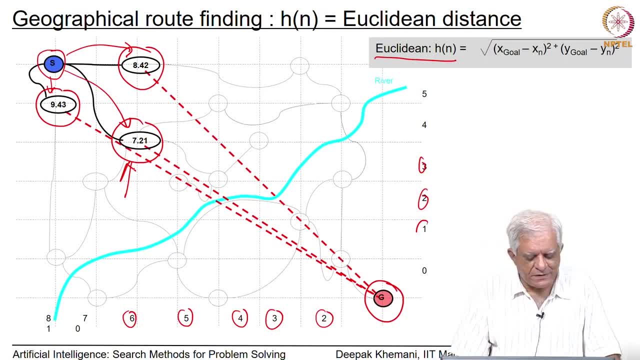 see that this also gives you a sense of direction. The problem is, the heuristic function is only looking at difference in coordinates, So it is not aware, for example, that there might be a river running across the path and the only bridges. So these two things which happen are here and here and here. but you know it will try. 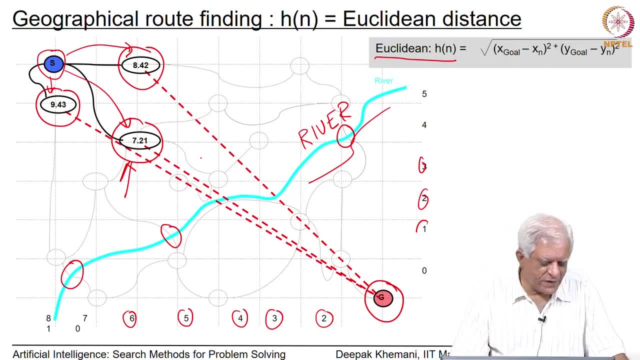 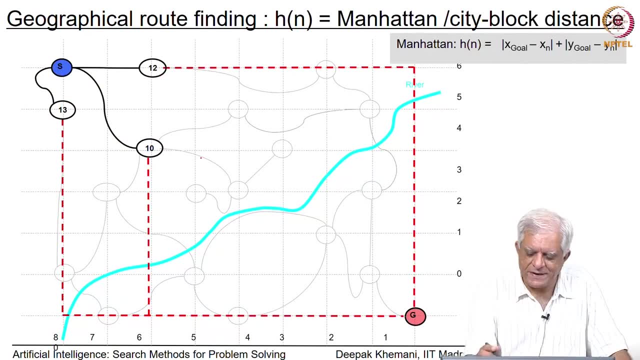 and drive you closer in the direction of the goal, and we will see a real world example in a moment. Another estimate of distance is the Manhattan distance, which, as you can see, simply the modulus of the differences of the x coordinates and the y coordinates. So this is called Manhattan distance because it is the kind 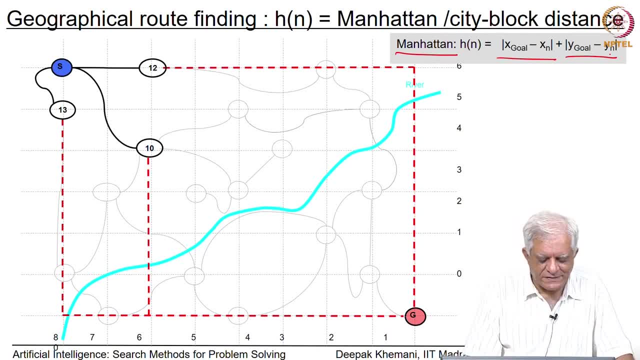 of distance You would have seen in a well structured town or city like Manhattan, where if you want to go from one point to another, you have to walk along one road, a certain number of blocks, and then walk along perpendicular direction. So the distance which you walk along is what? 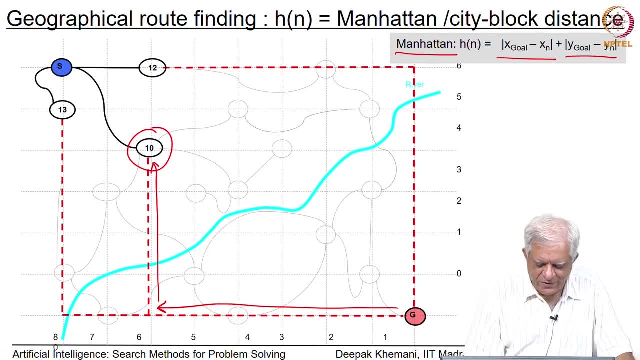 you count. So, for example, in this case the value is 10 because you walk 6 units this side and then 4 units up, and that is the estimate of distance. So this is 10, and this is 12, and this is 13 and, as you can see again, this also tells you that this node is a better 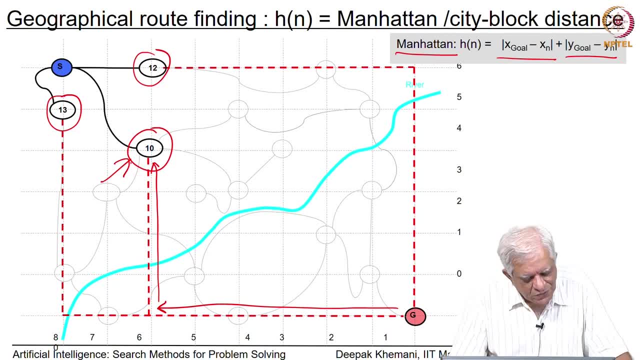 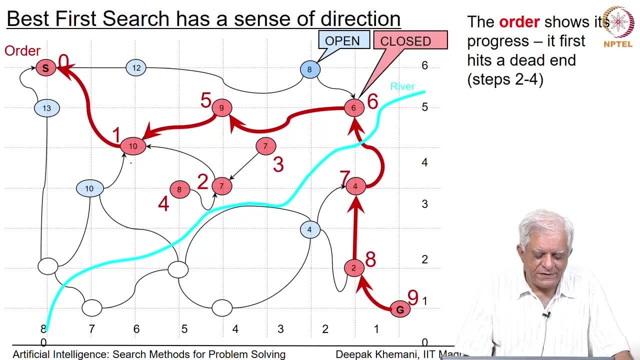 node to better node to go to Now. if you want to run best first search algorithm on this problem, then you would find that this is the kind of exploration it would have done. it will have the first node, or the 0th node would have been start then, as we just saw. 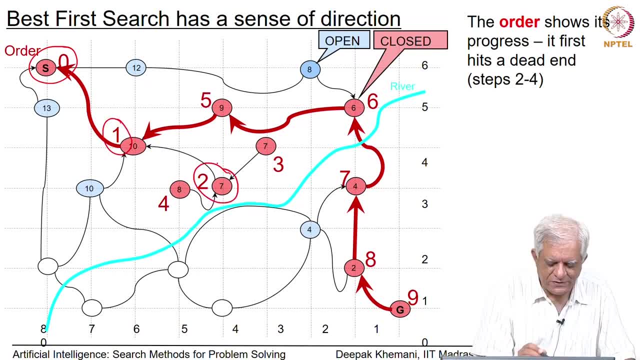 it would have gone to this node number 1, then it would have gone to this node because it appears to be closest to the goal, and then it would be forced to go here and then to node number 4 till after which, eventually, it finds a path through node, numbers, nodes, 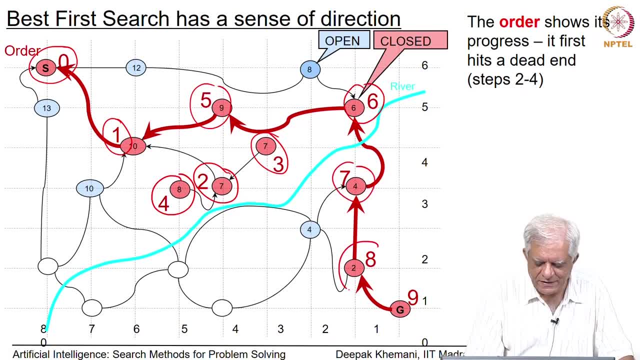 which is it sees in the 5th turn, 6th turn, 7th and 8 turn and this is the path that it is found to the goal. So this is the behavior of the best first search algorithm: it tries as far as possible to go towards the goal. but if 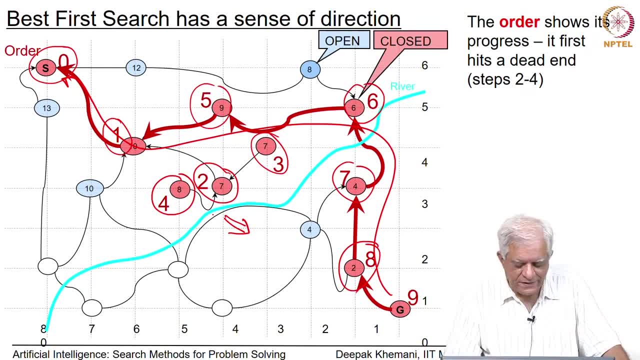 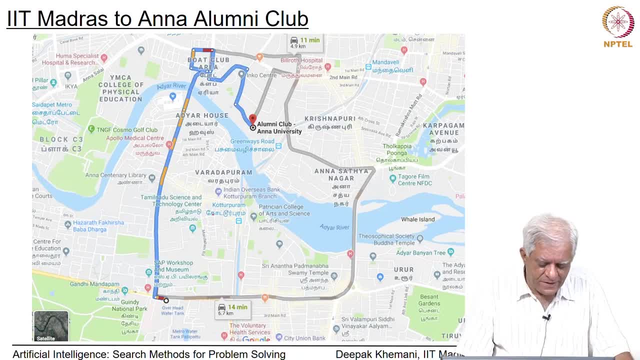 there is a obstacle on the way or, in this case, if there is a river, then you cannot. essentially, So here a real world example I was looking at a couple of days ago is that if you are here at IIT Madras and if you want to go to the Anna University alumni. 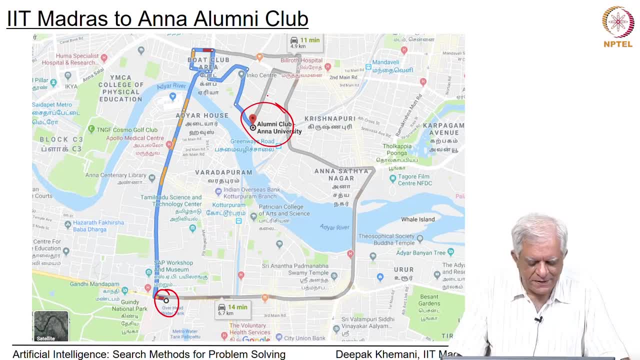 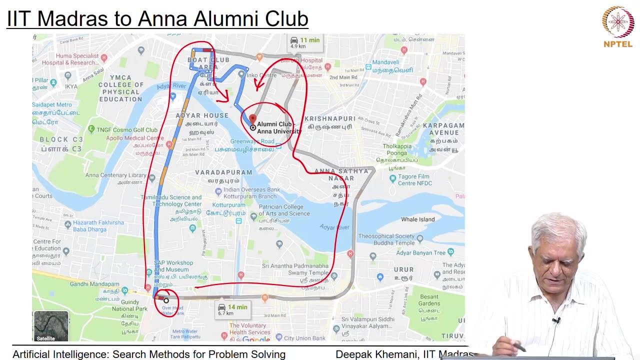 club which was hosting, which is in fact hosting a bridge tournament, and how do you get there? So, if you consult Google maps, then you can see that Google maps gives you this as the best path and it gives you some alternate paths which you can go, like this: 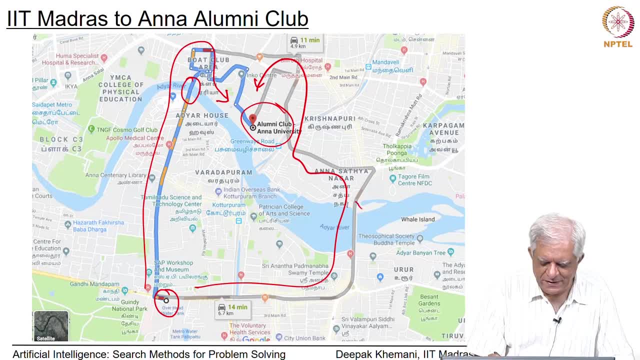 but it has figured out that there is a bridge here and there is a bridge here, So the path has to go through those bridges, and that is a thing that any search algorithm will do for you. as long as it is a global search algorithm, it will investigate all. 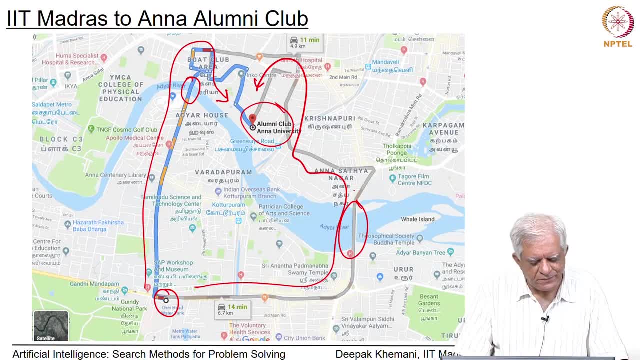 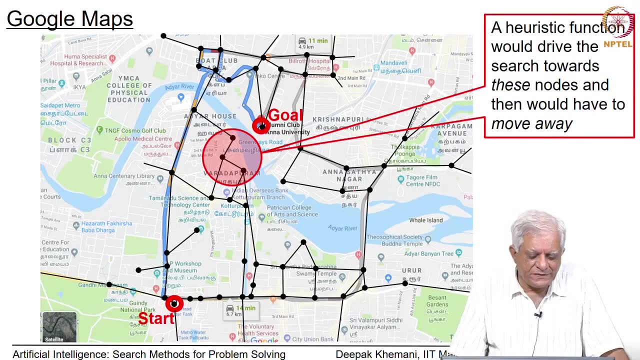 possible paths and take you to the path which it will find a solution for you essentially. Now, if you were to superimpose a graph on this same problem that we saw with this start node and the same goal In goal node, you will see that the search algorithm will drive you towards this set. 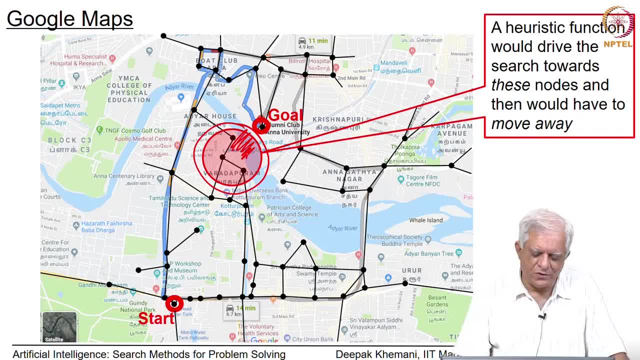 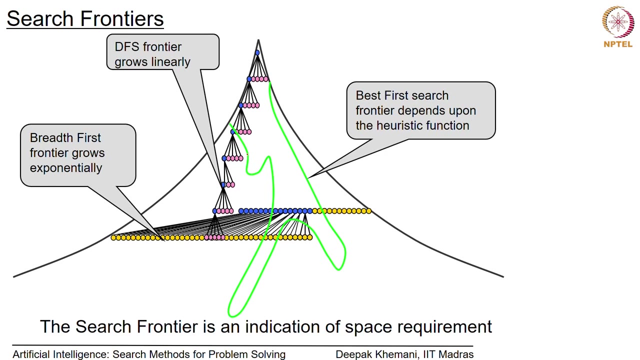 of nodes which appear to be closest to the goal node essentially. but because the algorithm is complete, because it maintains the open list- all other candidates that it has not yet inspected- it will eventually find the path to the goal node essentially. So how does the search frontier look like? We have already seen earlier that the search 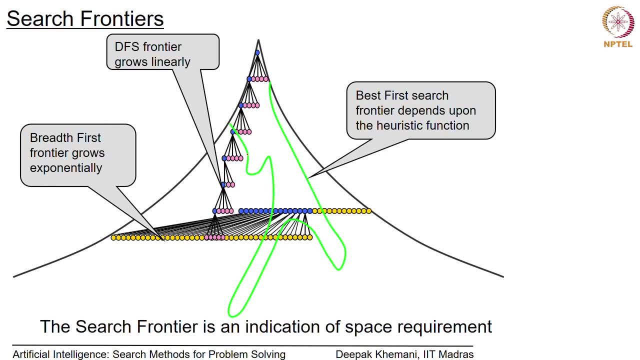 frontier for breadth first search is the set of pink nodes that we have, we are seeing here, which is going linearly. This search- frontier for breadth first search- was the set of yellow nodes that we have seen here In practice, because the performance of breadth 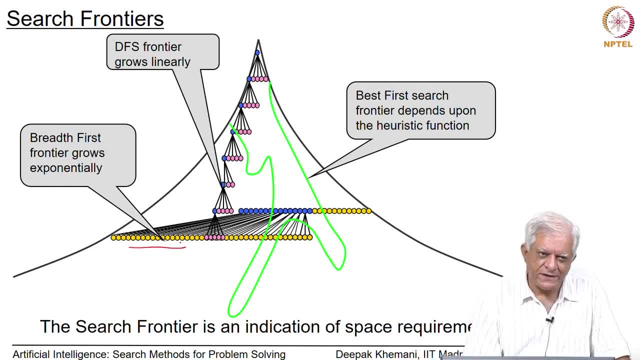 first search depends on the heuristic function and, as we have seen, that heuristic function can sometimes be misleading. it can take you towards the river front when you have to go from there somewhere else. So in practice the search frontier tends to be quite erratic. 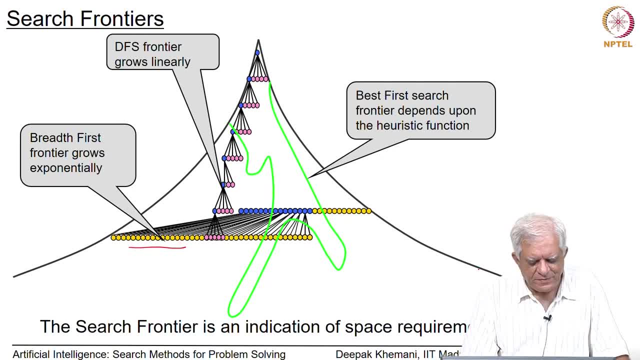 in nature, but it has been empirically observed that it is often tends to be exponential in nature. If you had a perfect heuristic function which is like an oracle which tells you what is the right choice to make at every place, then the search frontier would simply be linear. 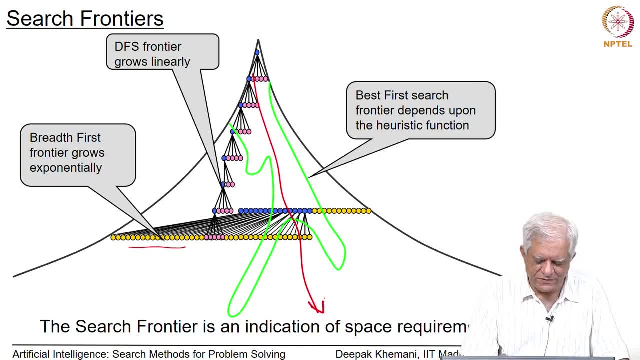 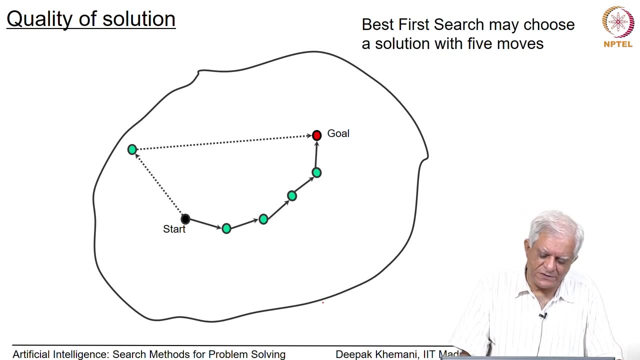 essentially, It will just go off in some direction, which takes you to the goal node, essentially. but unfortunately our heuristic functions are not perfect And hence the search frontier tends to be a little bit larger than a linear function. What about the quality of the solution found? So let us take this slightly contrived example. 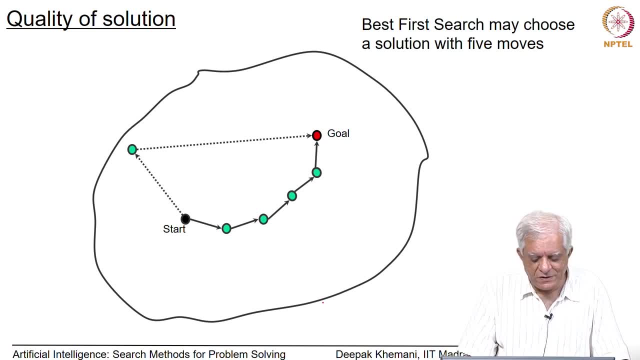 If you are at the start node here and you want to go to the goal node, then the. there are short segments of roads which take you to a path which is heading towards the goal, but the number of segments is 5.. 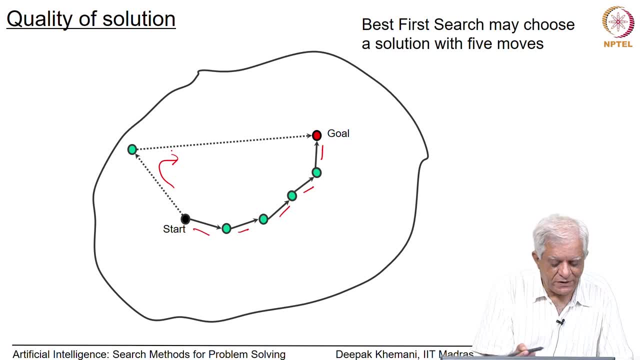 Whereas there is a longer way of reaching the goal, which has only 2 segments. So if you are interested in the number of hops, only then you can see that best first search does not find the shortest path. We will see variations of best first search, which will also give. 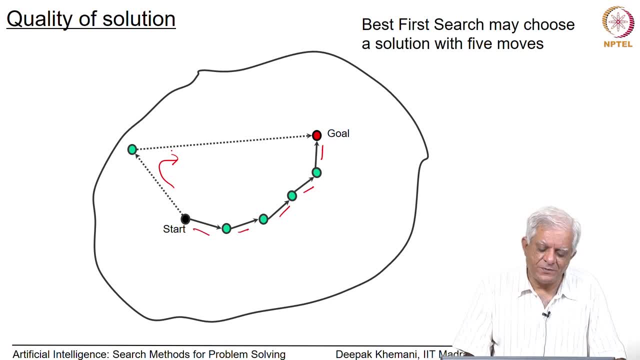 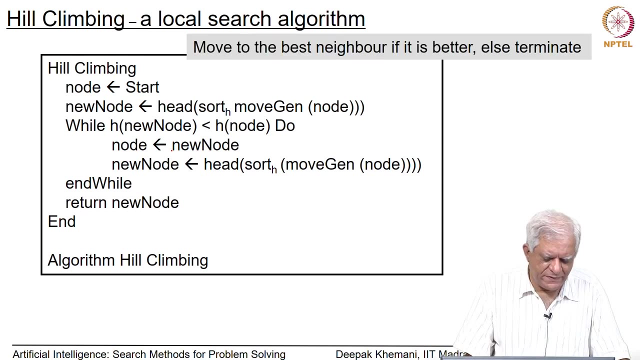 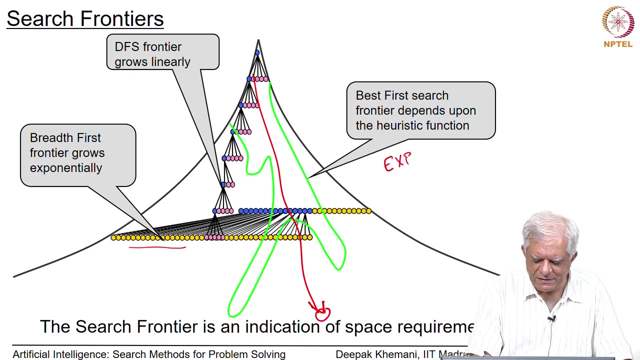 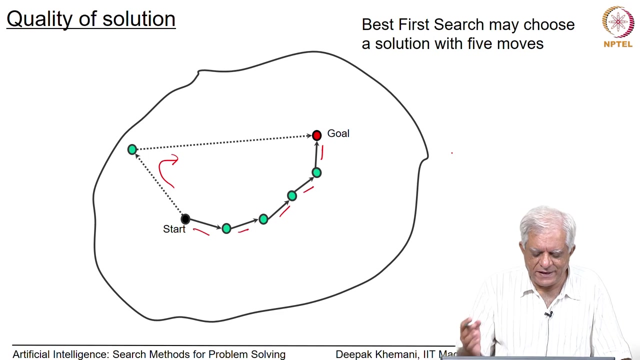 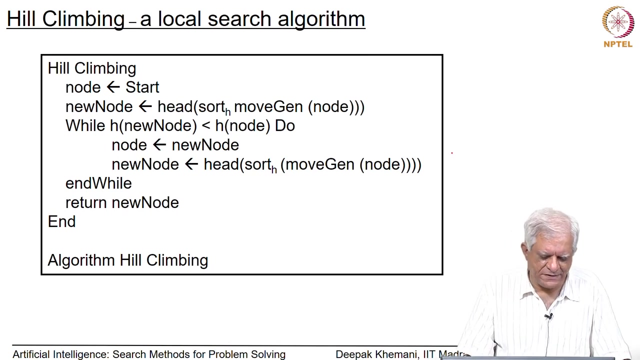 you shortest paths later, essentially, but at the moment we are focused more on finding the solution quickly, and that is what the heuristic function is trying to do for us. So this is seen as following that you are at some given node, which is initially the. 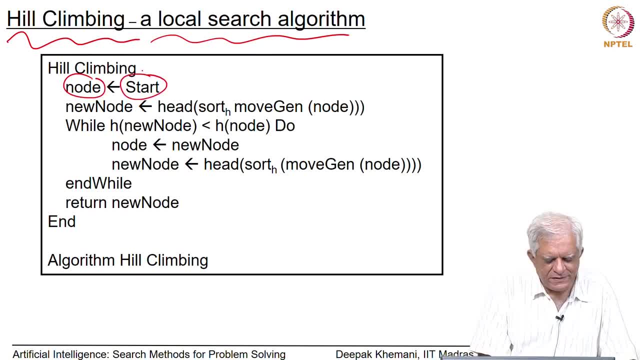 start node and you go to a neighbor which is the best of all its children, So you do move gen on that sort it pick the head. that is the best node. And if this new node is better than the old node, which is given by the fact that it is the heuristic value, 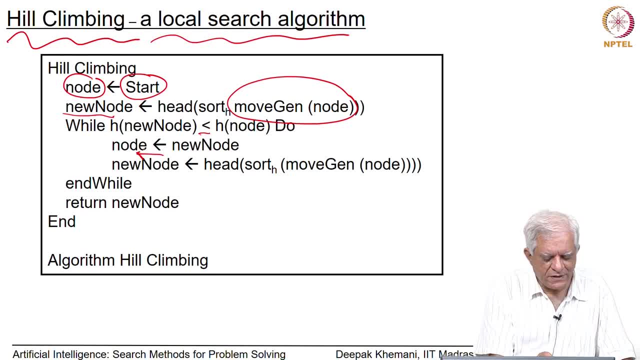 is less. you move to the new node which is shown here, and then look at the next node, which is one of the children of the or one of the neighbors of the node. So we just keep repeating this process of moving to the best neighbor if it is better, else you just stop batteryứomemberjizzus mud, feeling that the driver might not reach the targets, the judgment will be affected. the story might have notanas distinct, with the results being seen. so we just keep repeating. 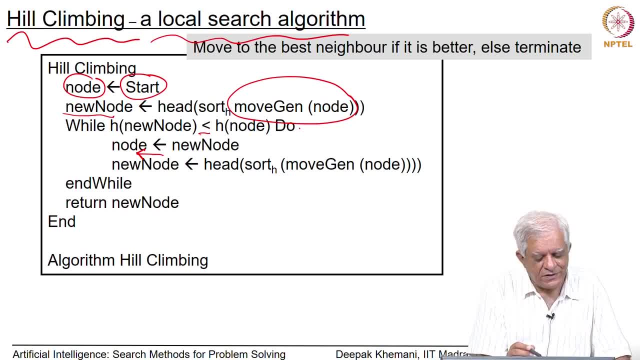 so while h of new node is less than h of node, you do this, otherwise you exit from there. in practice, you do not even need to sort the children of any given node, because sorting is still quadratic in nature, or at least n log n in nature, whereas you just want the. 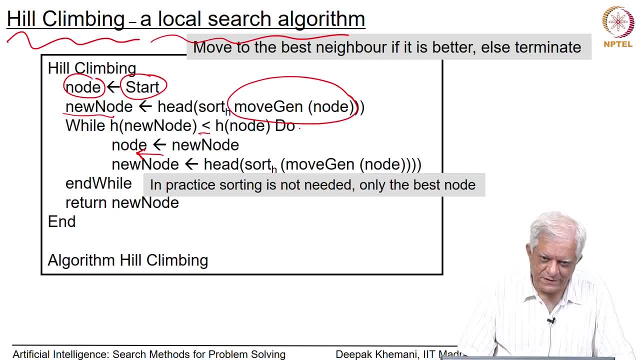 best node. so you can just scan it once and get the best node in linear time. but that is a matter of implementation we should not worry too much about. ok, one thing to notice is that there is a change in the termination criteria. we simply say that if you cannot, 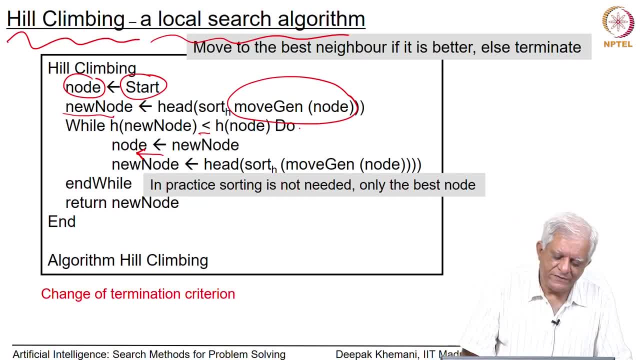 find a better node, you terminate. which is very different from what we said earlier is that if you have found a goal node, you terminate, or if there is no path to the goal node, then you terminate. here it is neither. it simply says: if you cannot find a better node, 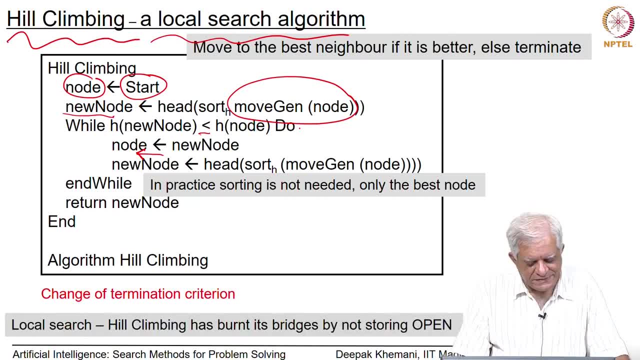 you terminate and that we will see results in certain change in behavior. The point to note is that, as a local search algorithm, it has burnt its bridges by not storing the open list, So it can go and go and get stuck in the local optima. The nice thing about hill climbing is that it is a constant space algorithm. 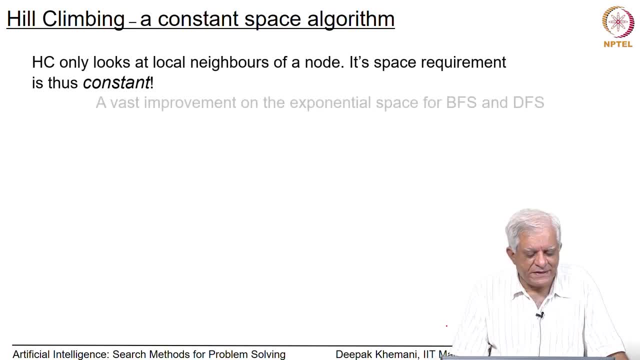 it only looks at the neighbors of the node. Its space requirement is thus constant, which is a vast improvement on the exponential space for breadth first search and breadth first search that we needed. overall space requirement It is. behavior is that it only moves to a better node, which means it will terminate if it cannot move to a better node. So 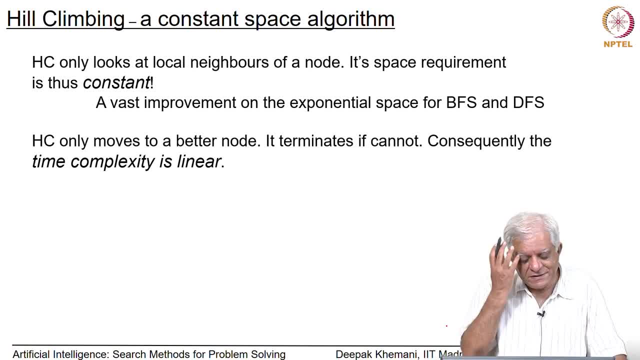 consequently, its time complexity is linear in the, in the depth, essentially that it goes to a certain distance and stops, and you know, but it does not spend time looking here and there. Its termination criteria, as we just mentioned, is different. it stops when, no better. 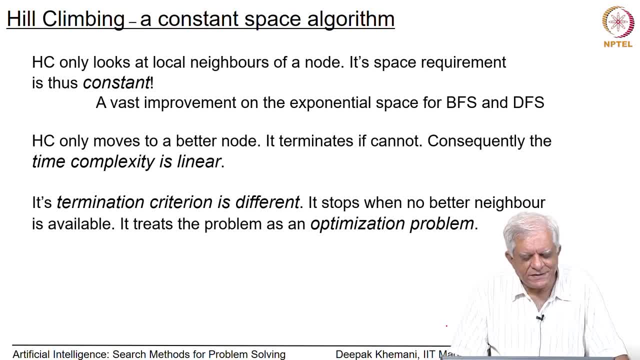 neighbor is available. So in some sense it reads the problem as an optimization problem. it says: give me the best value of h that you can find, instead of saying give me a path to the goal, essentially. So it is like thinking of it as an optimization problem, and it is. 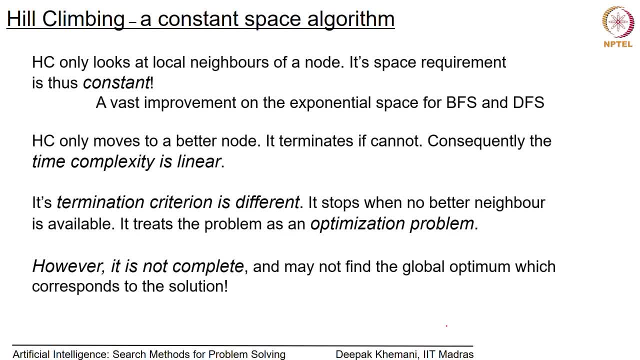 not complete, essentially, as we will see that it may not find the global optimum which corresponds to the solutions. So if we remember the eight puzzle example and the city map example that we considered the little while ago, you would notice that hill climbing would have, you know, stopped much before reaching the goal. So hill climbing, 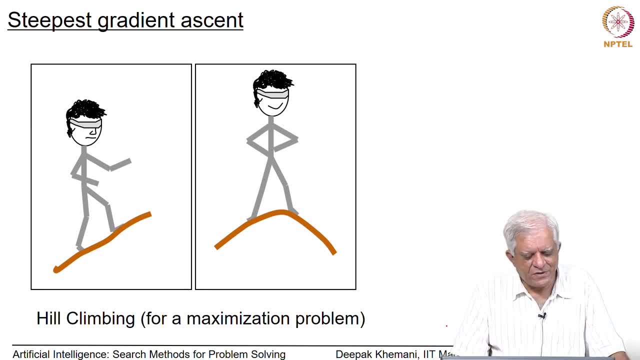 is also known as the G70. steepest gradient algorithm, or gradient descent algorithm, or gradient ascent algorithm, as the case may be. It really depends on whether you want to maximize the heuristic function or minimize the heuristic function. And if you think about this maximization and 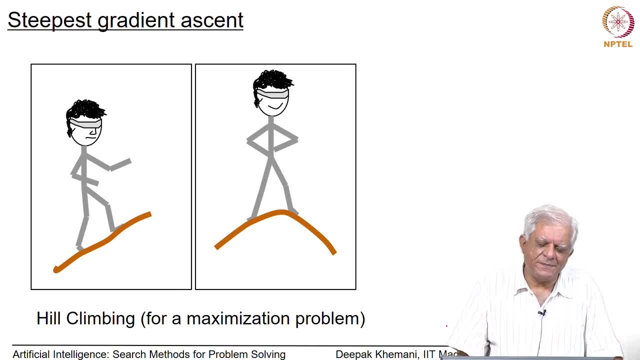 minimization are just two sides of the same coin. So in the eight puzzle, for example, if you want to minimize the number of tiles which are out of place, it is equivalent to saying that: maximize the number of tiles which are in place. essentially, 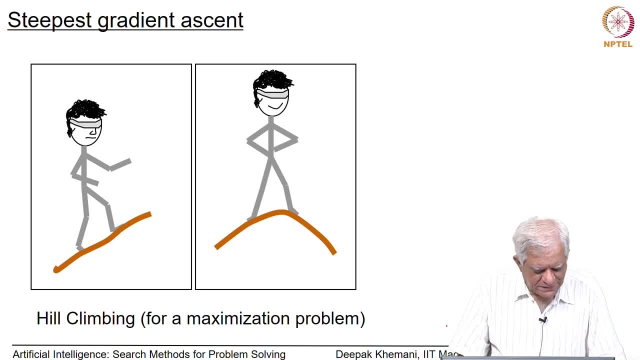 So if you are talking about the maximization example, then hill climbing is essentially saying that you go in the direction of the steepest gradient, you just keep climbing and you stop climbing when you have reached a point where no neighbor is better than another. 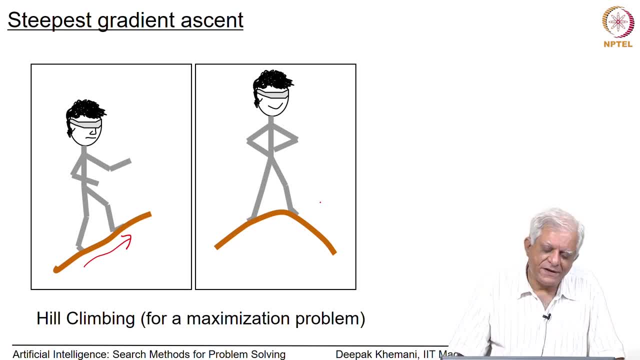 neighbor. Now, as you can imagine, if you are doing this, if you are blinding yourself, you are not going to be able to see the whole picture. So if you blindfolded and put on a hillside and you would do something like this and not, 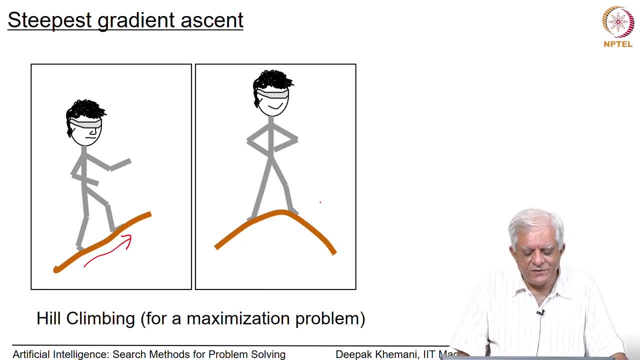 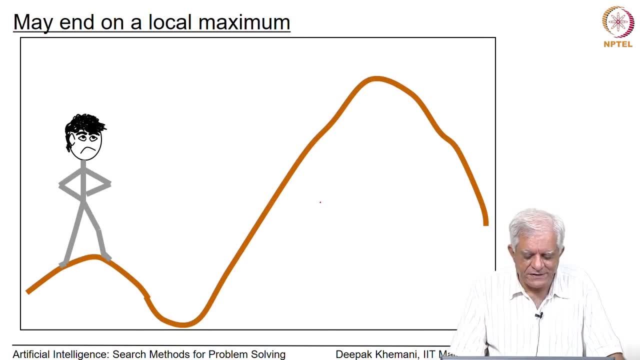 surprising with this algorithm is called hill climbing. you would reach a place where you thought was the top, but if you were to open your eyes, you would see that it is what is called as a local maximum And you have not found the solution, but the algorithm will. 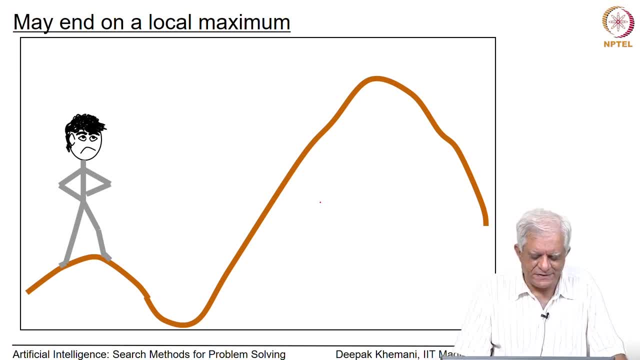 terminate at this place, essentially. So what do we do? We can single pick the ignition to limit term würdeгля series, And so, by thinking about the typical receives, step one, we can breaker it. if I am working in a city like 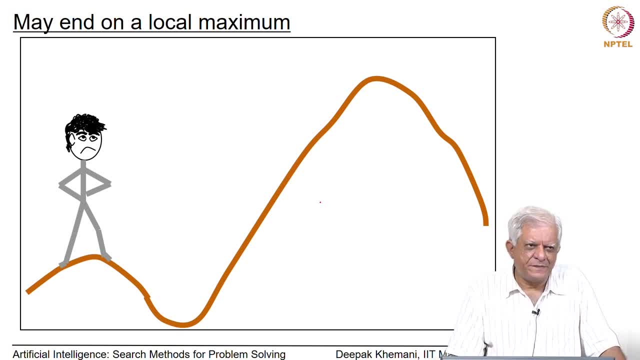 that we somethin also knows that skipping the lights and turning on a light in the mooring for the second figure, Yes, Yes, we fit when the play is applied to a larger area, but we are going toMO. This is something problem that we do in the next few classes. We will start off by looking.